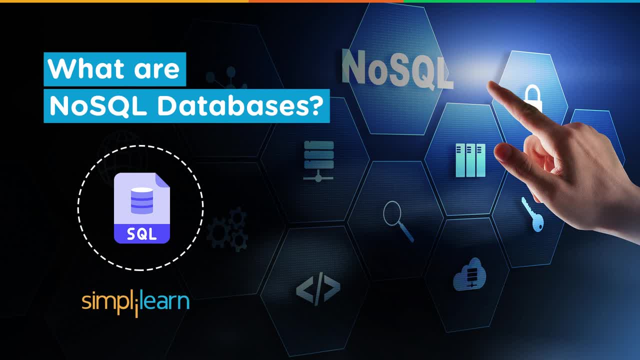 possible. In today's session, we'll be going through NoSQL database and we'll understand what exactly are NoSQL database, how they came into existence, why we use them and how they are different from traditional non-relational databases. Let us just wait for another two. 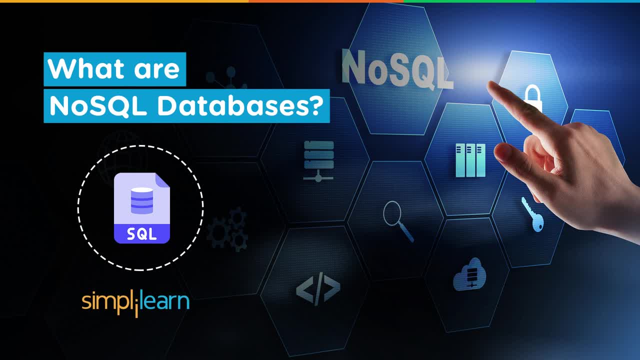 minutes, so that rest of the people will also join this session. In the meantime, guys, I would like to update that we have regular updates on multiple technologies on our channel, So if you are a tech geek and love watching tech videos, consider getting subscribed to our channel. SimplyCode to. 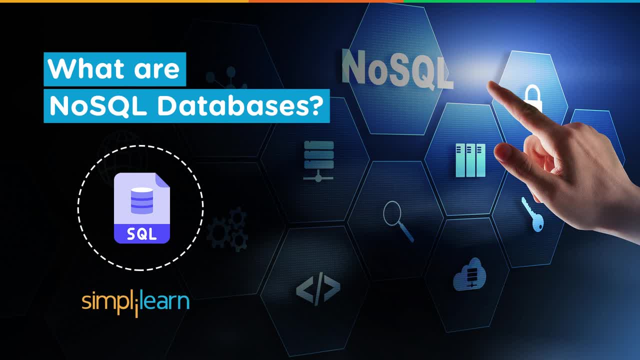 stay updated with all the latest technologies. Hit the bell icon to never miss an update from us. Alright, as you all know, we're living in the era of big data, where massive volumes of data are generated per second worldwide. So handling and storing these huge chunks- 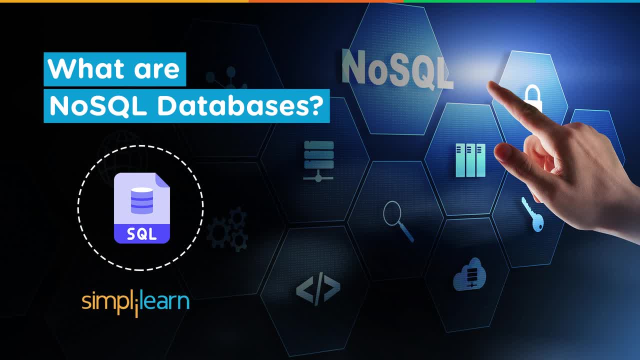 of data is pivotal and paramount for all the companies around the world. Traditionally, relational databases were used to store this data prior to when the internet came into existence. Now, in the early 1990s, the internet gained extreme popularity and the relational 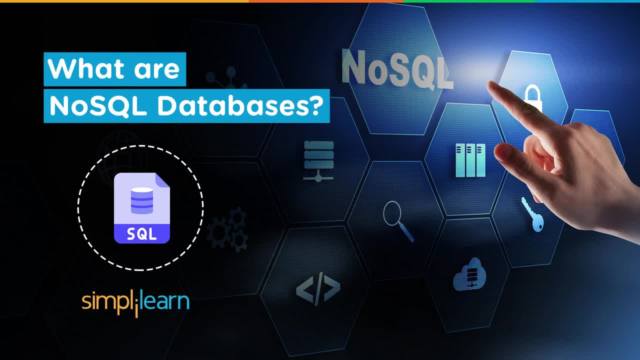 databases could not keep up with the flow of information and data demanded by the users, as well as the large variety of data types that occurred from this evolution. This led to the development of non-relational databases, often referred to as NoSQL. The not only SQL, or commonly known as NoSQL databases is an approach to data management. 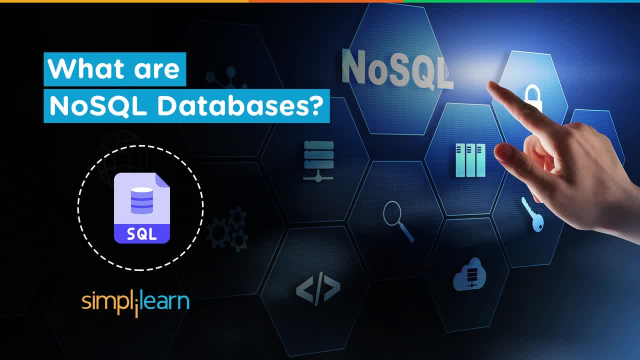 and database design that may be useful for large sets of distributed data and unstructured data. It basically consists of a collection of technologies and architecture that seek to address big data, performance and scalability- issues that relational databases cannot address. So this database is used when businesses and enterprises require access to and analysis. 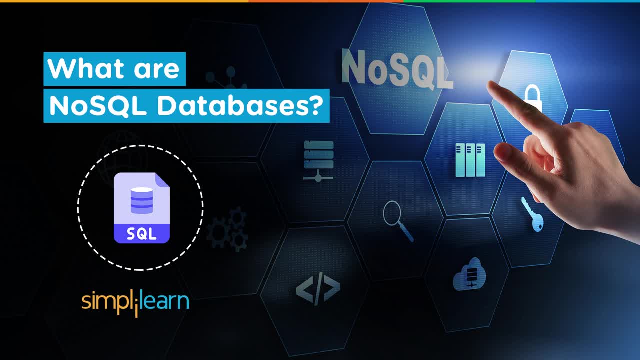 of large amounts of unstructured data. Now, this unstructured data can be of any type. It can be a text file, it can be an image or video and others that are stored across multiple servers. So it is important to know that this data can be of any type. 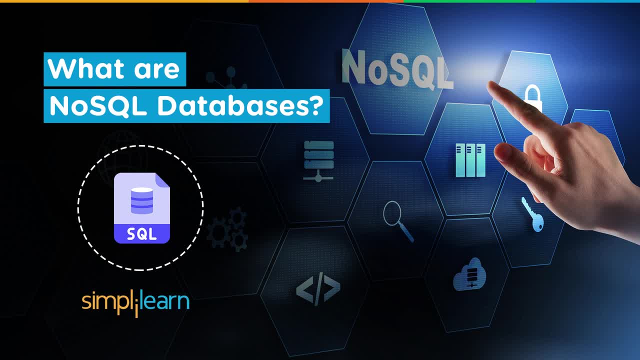 It can be a text file, it can be an image or video and others that are stored across multiple servers. It is important that we understand how this NoSQL databases work, so in today's session we will be going through all the concepts that are needed to understand what NoSQL databases 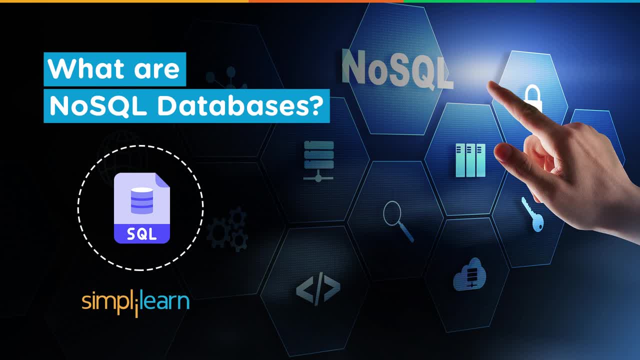 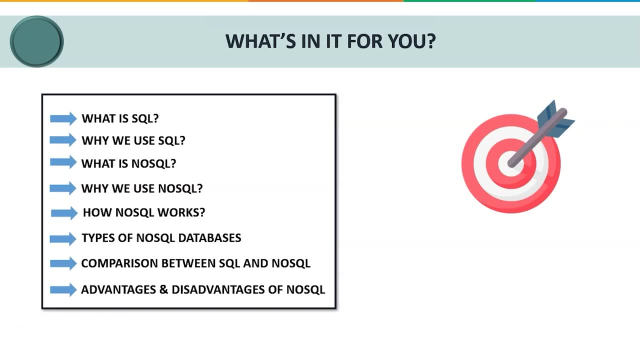 are and how they exactly work. So, without any further delay, let us jump straight into today's topic. Firstly, let us go through the agenda for today's session. We will start the tutorial by understanding what is SQL, and then we will look at why we. 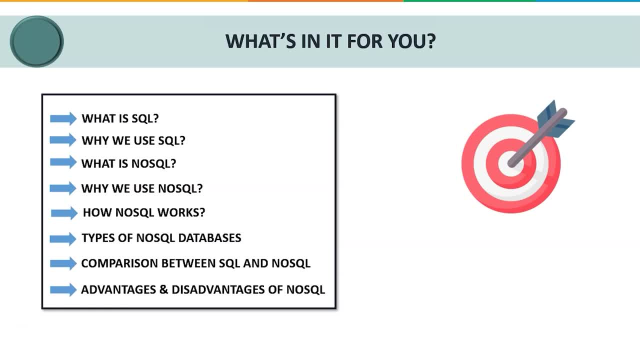 use SQL, and after that we will understand what is NoSQL databases database, and then we'll understand why we use NoSQL. Up next, we'll understand how to use NoSQL and how exactly it works, And then we'll look at some different types of NoSQL databases, and after that we'll have 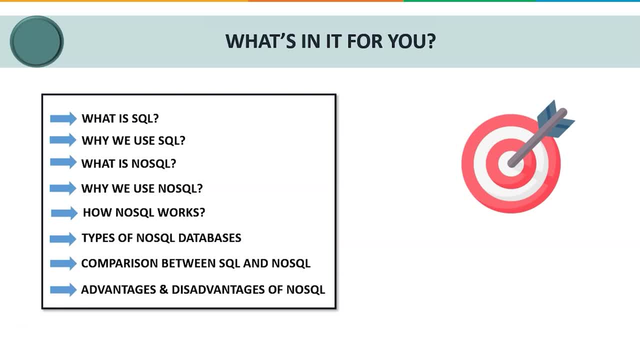 a detailed comparison between SQL and NoSQL database. and finally, we'll conclude the session by understanding some advantages and disadvantages of using NoSQL, and we'll also look when to use SQL as well as NoSQL. So, without any further delay, let us dive straight into today's topic on SQL vs NoSQL. 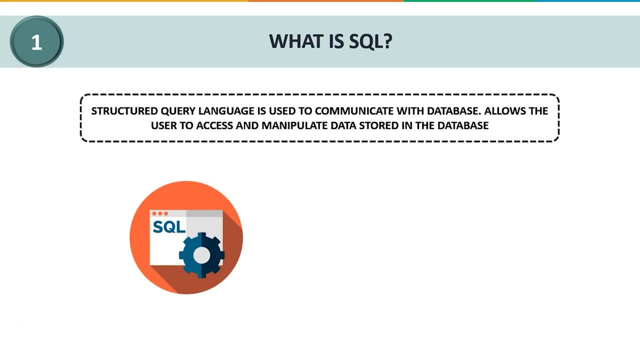 Firstly, let us understand what is SQL. SQL, as it stands, is defined as Structured Query Language, is basically a standardized programming language that is used to manage databases, and it performs various operations on data in them. Initially created in 1970s, SQL is widely used by many companies and technologies nowadays. 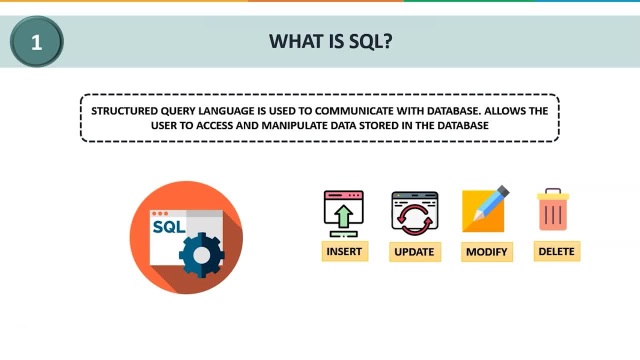 SQL is used for modifying database tables and index structures. It is also used in adding, updating and deleting rows of data. It is also used to retrieve subsets of information from within the database management system. Now SQL is used to perform various actions, such as to insert data, to update data, modify. 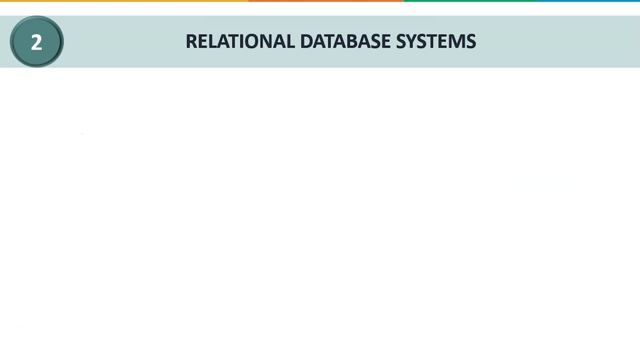 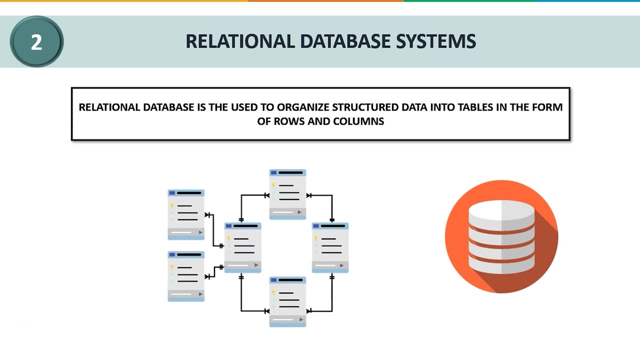 and delete the data in the database as well. Now, when we talk about SQL, it is important that we talk about relational database systems as well. A relational database system, or RDBMS, is a database system. A relational database system, or RDBMS, is a database system. 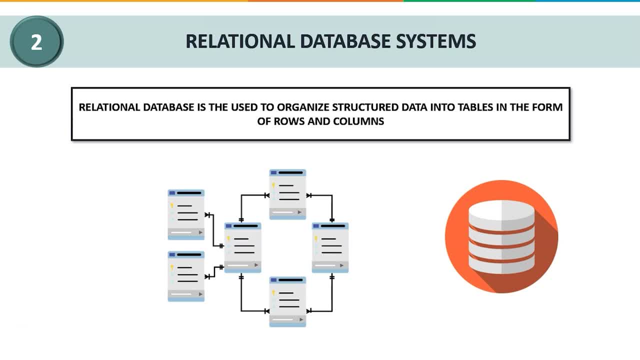 A relational database system, or RDBMS, is a database system. A relational database system on SQL is designed to積 up and plenty align those other components in a system that stores and fetches data in the form of a table, that is, in the form of rows and columns. 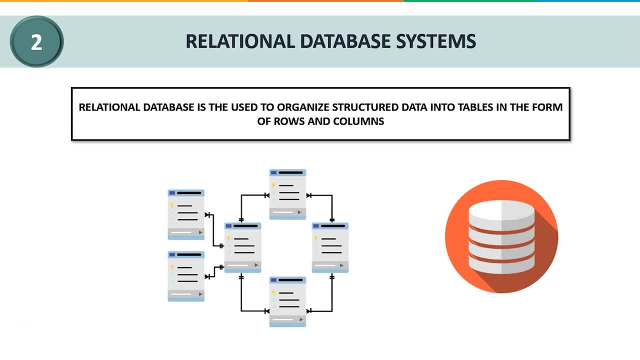 Tables are used to store data and relational databases about related objects. Each column contains attributes of data, whereas each row holds a record of unique data, known as a key, which helps in making a relationship between different data points that is present in different tables, which makes it easy to understand. 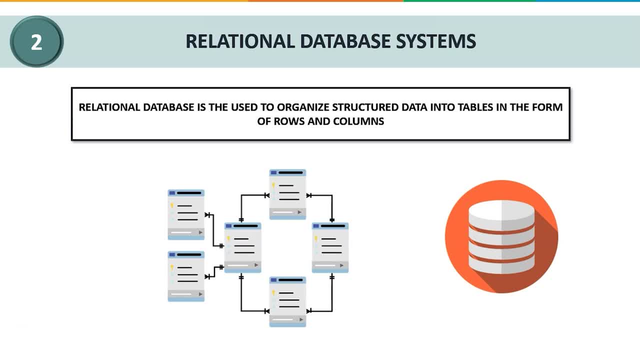 These relational databases, or RDBMS, are managed using SQL language to perform variousrittable, various operations. Therefore, SQL codes are used to retrieve information from these relational databases by doing various interactive operations like using join, create, truncate, delete, alter and etc. 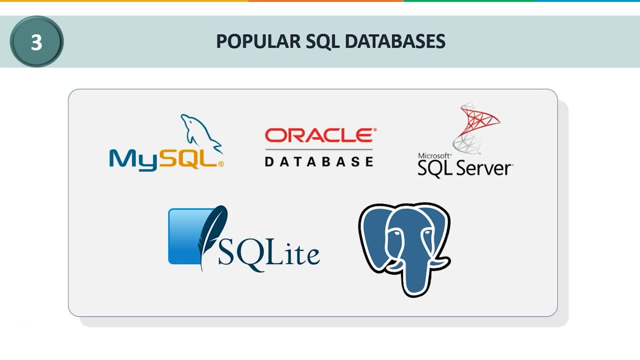 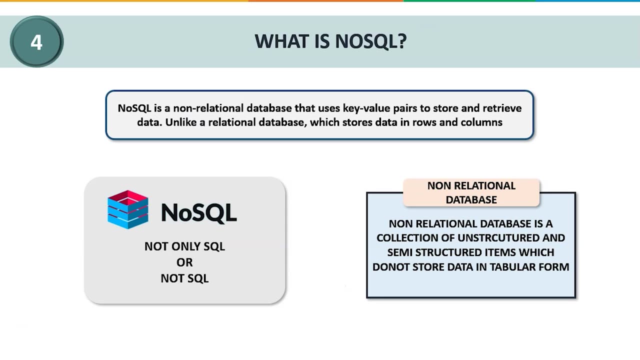 Let us now look at some popular SQL databases. Some popular SQL databases that are available are MySQL, Oracle Database, Microsoft SQL Server, SQLite and PostgreSQL. Now that we have understood what is SQL, let us now understand what is NoSQL. NoSQL database is a non-relational database management system that does not require a fixed schema, ie the data is not stored in the form of tables in NoSQL databases. 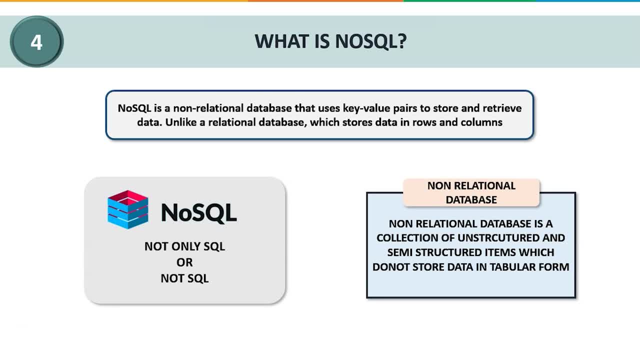 Basically, it avoids any joining, creating or scaling the databases in SQL. The major purpose of using a NoSQL database is for distributed data storage, which is having high volumes of data storage needs. NoSQL is used for big data and real-time web applications. For example, companies like Amazon, Facebook, Google collect terabytes of users' data every single day. 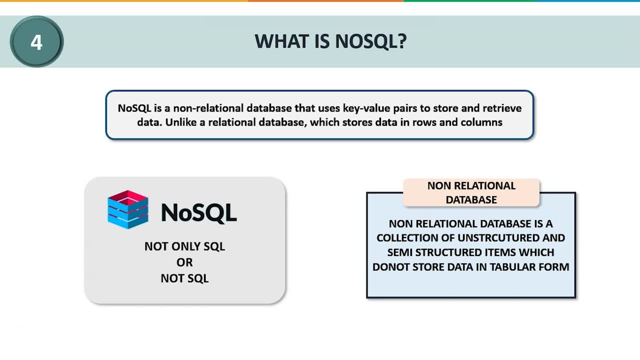 Basically, NoSQL database stands for not only SQL or not SQL, and it is introduced in the year 1998 by Karl Strauss. Traditional RDBMS uses SQL syntax to store and retrieve data for further insights Instead. a NoSQL database system encompasses a wide range of database techniques. 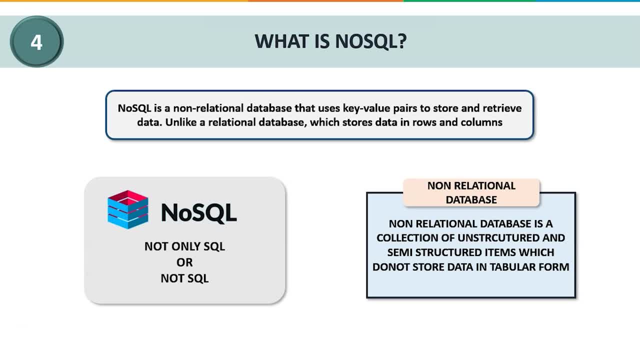 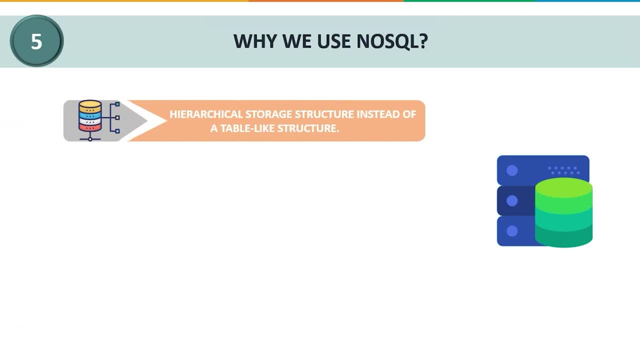 It can store structured, semi-structured as well as unstructured data. Let us now understand why we use NoSQL. We use hierarchical storage structure instead of a table-like structure. That means before relational databases, companies used a hierarchical database system with a tree-like structure for database tables. 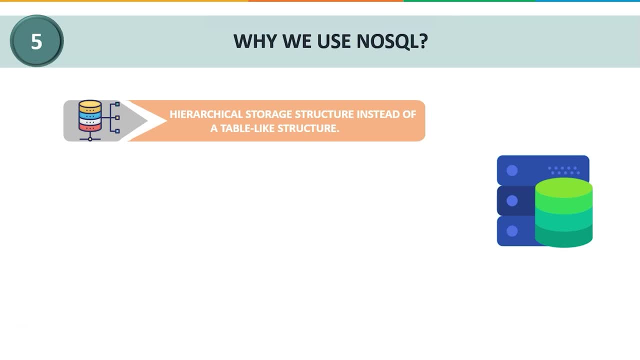 These early database management systems enabled users to organize large quantities of data. However, they were complex, often required a particular application and in a limited way which they could uncover the data that is stored Now. these limitations eventually led to the development of relational database, that is, the data that is stored in tables. 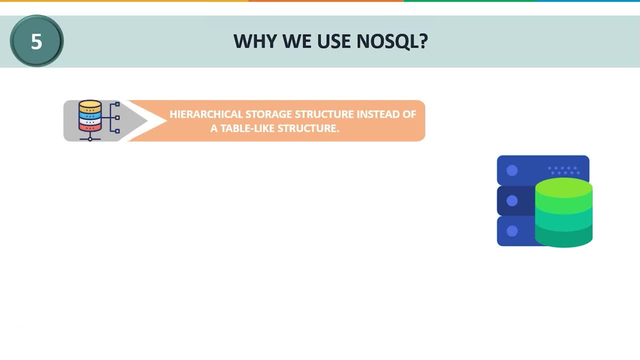 So SQL provided an interface to interact with relational data, allowing the analyst to connect tables by merging on common fields. But as time passed, the demand for faster and more desperate usage of larger datasets became increasingly more important for emerging technologies, for e-commerce and other big giants. 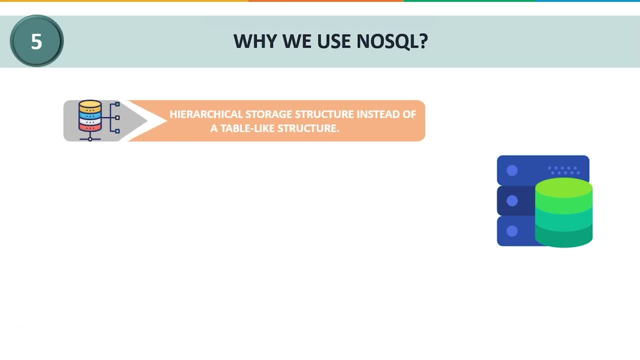 For that, NoSQL has become the alternative for everyone. Another reason is that we now have constant addition of new features and functions in the NoSQL database. That means we know that technology is rapidly evolving and huge amounts of data are being released on a daily basis. 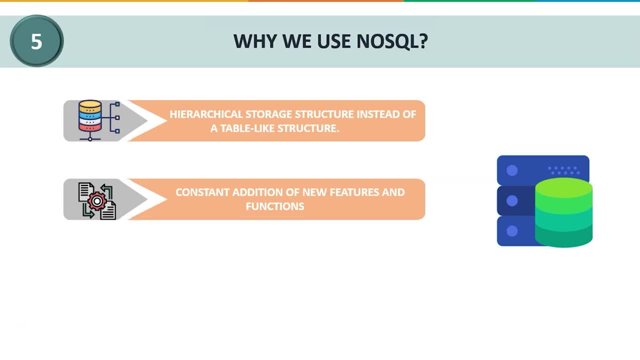 And it's important that we store this data and access in a quick way Now. NoSQL is the best database to use for large amounts of data or for ever-changing datasets. It is also best used when you have to have a flexible data model or need that don't fit into a relational model. 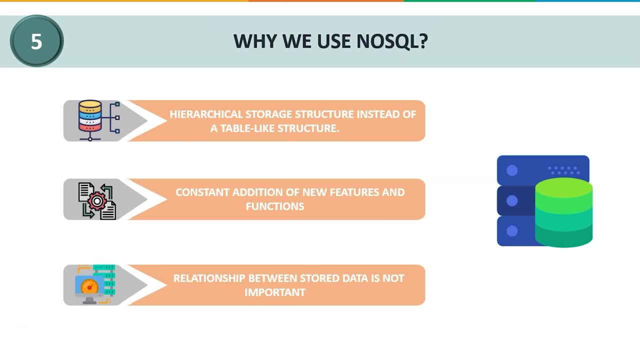 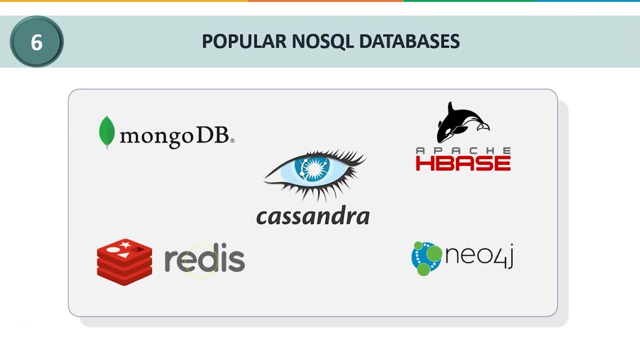 And finally, if you want that there is no relationship between any stored data and you feel it is not important, then you can use NoSQL as well. Let us now look at some popular NoSQL databases. Some popular NoSQL databases are MongoDB, Apache, HBase, Cassandra, Redis, Neo4j and etc. 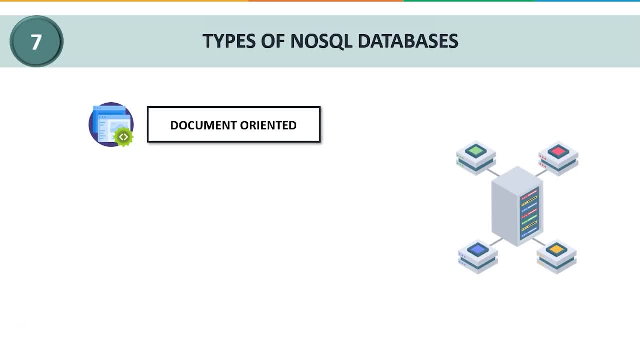 Let us now look at some types of NoSQL databases that are present. Firstly, we have document-oriented. The document database typically stores self-describing JSON, XML and BSON documents. They are similar to key-value stores, But in this case a value is a single document that stores all the data related to a specific key. 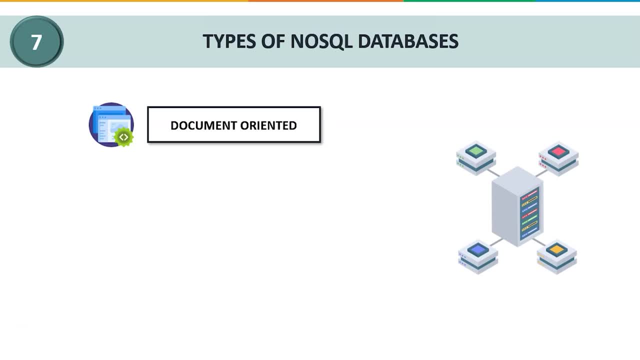 Popular fields in the document can be indexed to provide faster retrieval without knowing the key. as well, Each document can have same or different data structure. MongoDB, CouchDB, Cloudant are some examples of document-based NoSQL databases. Next, we have key-value pair database. 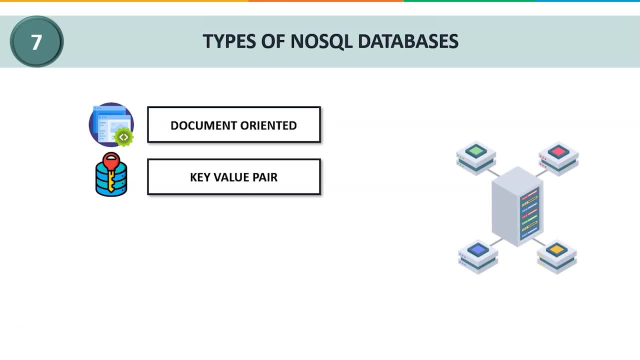 The data in this is stored like a key-value pair. Key-value pair data stored in database in the form of a hash table. Each key is unique. in this case, The value stored may be an integer string, a binary object, a JSON object, etc. 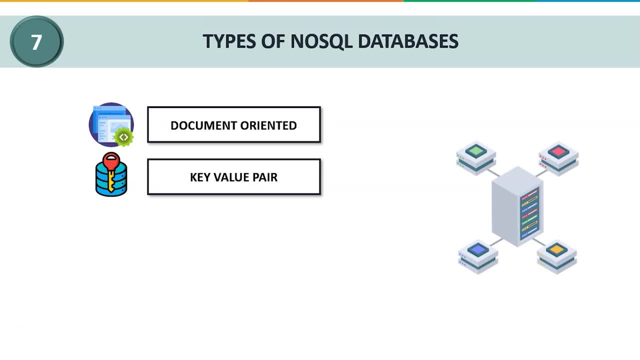 The key-value store based database is simplest database among all the databases in NoSQL database, Redis, Coherence are examples of some key-value stored databases. Next we have column-based or column-stored database in NoSQL, Which is, in this, the data stored in group database. 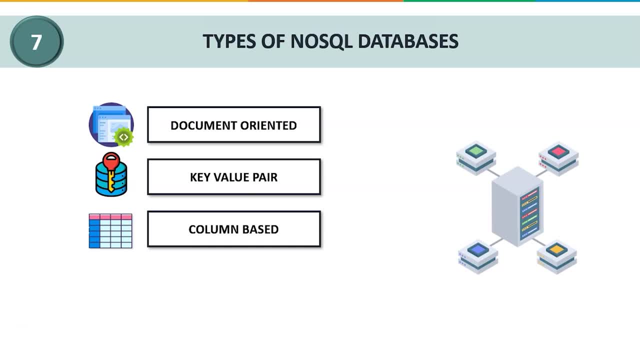 It is grouped to columns instead of rows. Every column values are stored separately. It delivers high performance on aggregate functions like count, sum, max minimum. Group of columns are data stored in key spaces, like schema in RDBMS. Key spaces contains group of rows or columns. 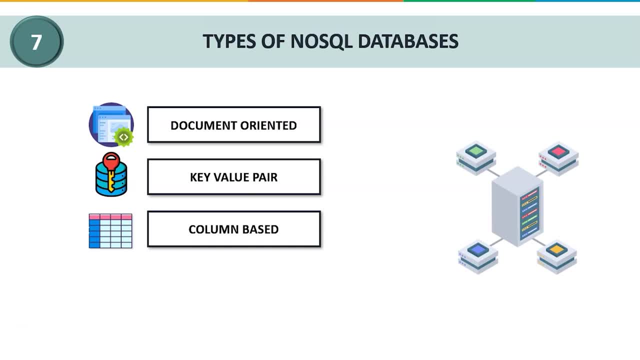 And HBase, Bigtable, Aculamo are some examples of column-stored databases. And finally we have graph-oriented or graph-stored databases. Data in this is represented in the form of a directed graph. It consists of nodes and edges. 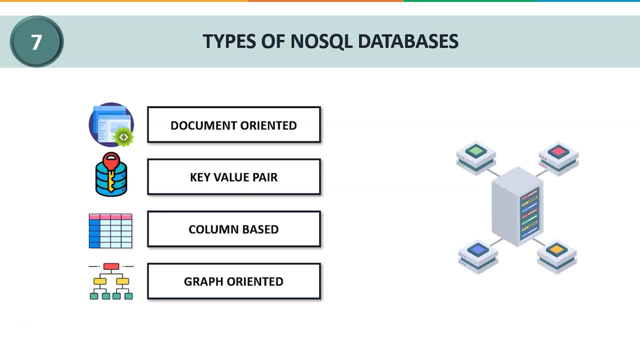 Nodes represent an entity and any edge represents the relation between the two nodes. Node edge to be unique. Social networks, logistics, PATL data used. graphical storage database. Neo4j, Infinite Graph, OrientDB, FlockDB are examples of some graph storage database. 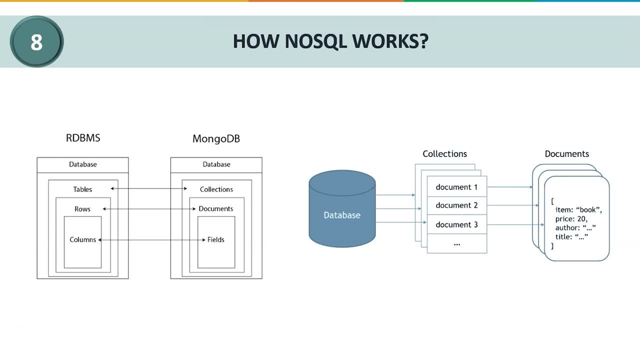 Next, let us understand how exactly NoSQL database works. For that, I am going to take the example of MongoDB database Now. MongoDB is based on the NoSQL document store model, in which data objects are stored as separate documents inside a collection instead of a traditional column and row of a relational database. 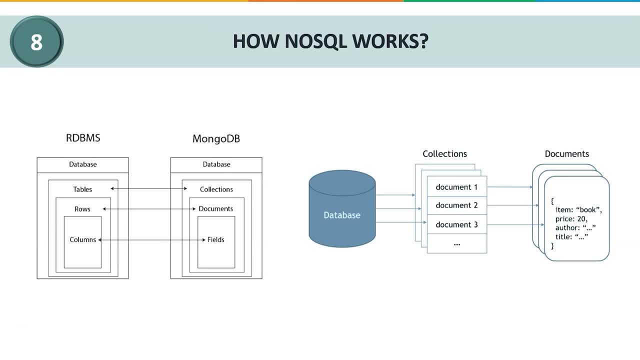 Now MongoDB groups data through collections And basically a collection is simply a grouping of documents that have a same or similar purpose. A collection acts similarly to a table in a traditional SQL database. However, it has a major difference. A collection is not enforced by a fixed schema. 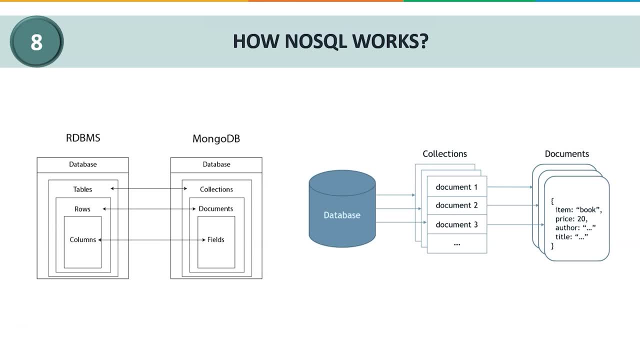 That is, it does not have any fixed schema at all. Instead, documents in a collection can have slightly different structure from another, as needed. This reduces the need to break items in a document into several different tables, as it is often done in an SQL implementation. 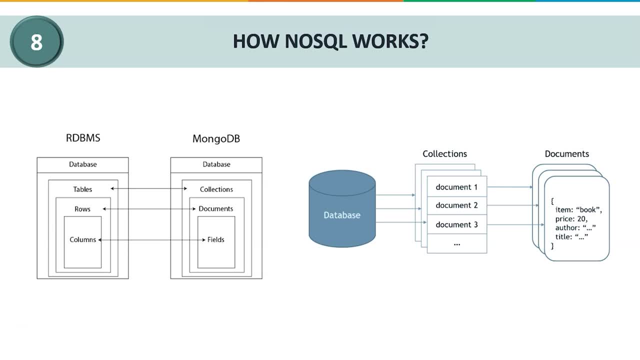 Now coming to document. a document is a representation of a single entity of a data. in MongoDB database, A collection consists of one or more related objects. A major difference that exists between MongoDB and SQL is that in that, documents are different from rows. 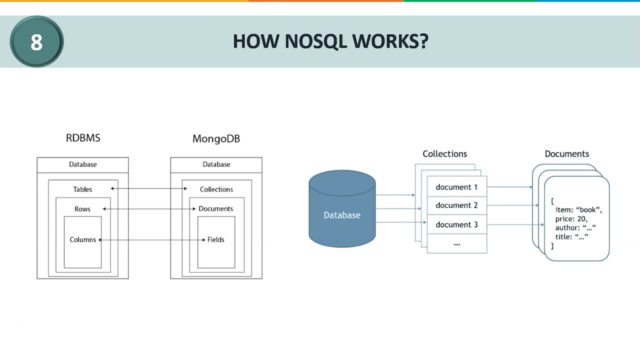 Row data is flat, with one column for each value in the row. However, in MongoDB, documents can contain embedded sub-documents, providing a much closer inherent data model for your applications. Now, if I just have to map what are exactly and how it is different from RDBMS. 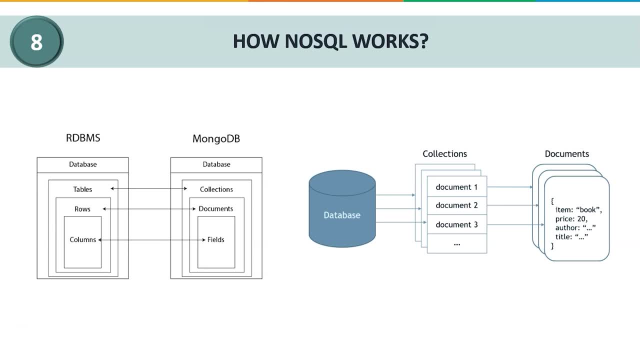 A collection in a MongoDB is equivalent to the tables in RDBMS And a document in MongoDB is equivalent to the rows And fields in MongoDB is equivalent to the columns in RDBMS. So this is how a document looks in a MongoDB. 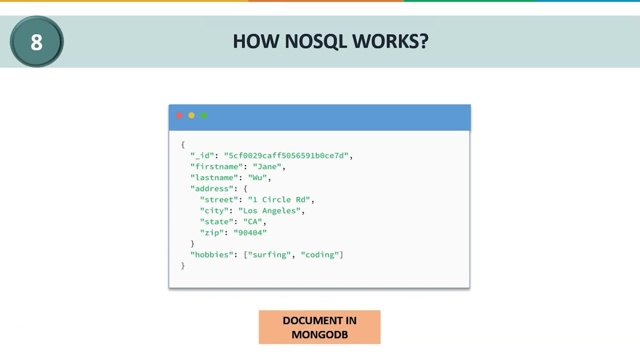 As you can see, this is similar to a row in RDBMS, but we just have a field and a value that is taken separately instead of a tabular value. And another important thing to note here is that MongoDB supports dynamic schema, which means one document of a collection can have a number of fields, while the other document can have less or same number of fields. 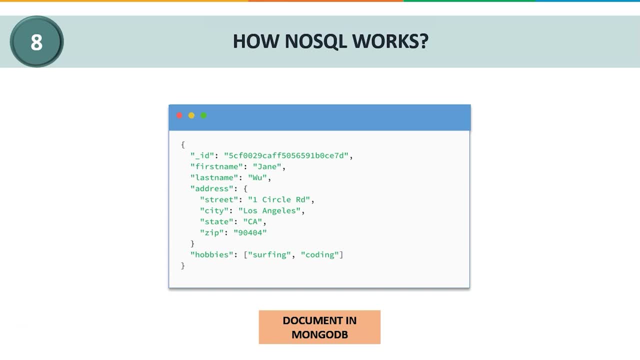 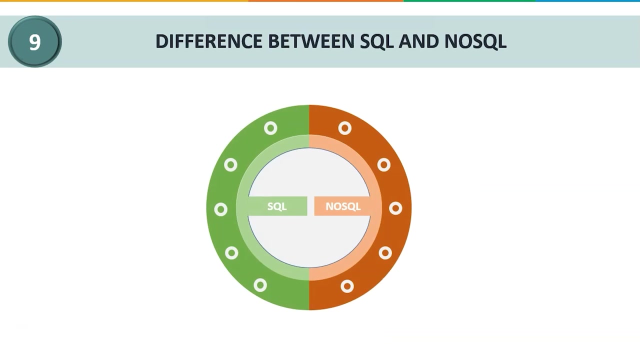 That is, if a collection can have four fields while other document can have only just two fields, Which is basically not possible in a relational database which does not exist as it does not support, because it needs a particular and a fixed schema. in that. Let us now understand some differences between SQL and NoSQL. 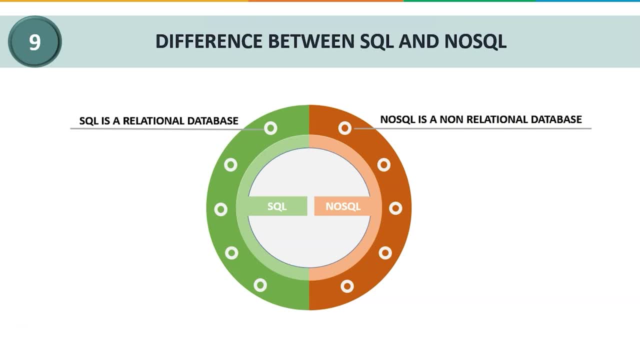 Firstly, SQL is a relational database and NoSQL is a non-relational database. That means SQL databases are in the form of tables that can contain rows and columns and they have fixed logical schema design. All the data in SQL is arranged in tabular format and it is well suited for complex queries. 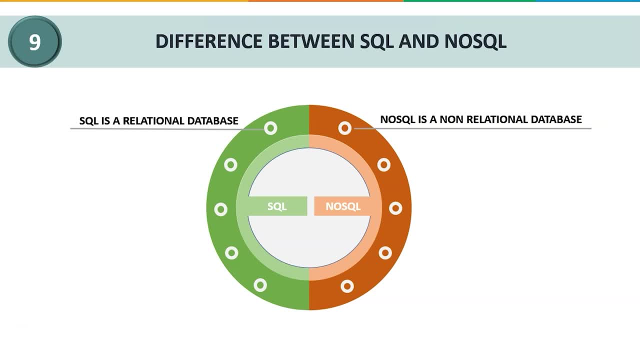 And, on the other hand, NoSQL databases is a non-relational database. That means it does not store data in the form of tables and contains collections, And inside every collection there is a document that contains the data of a single entry. This data is stored in the form of a key-value pair, unlike SQL, where we store data under the fixed schema. 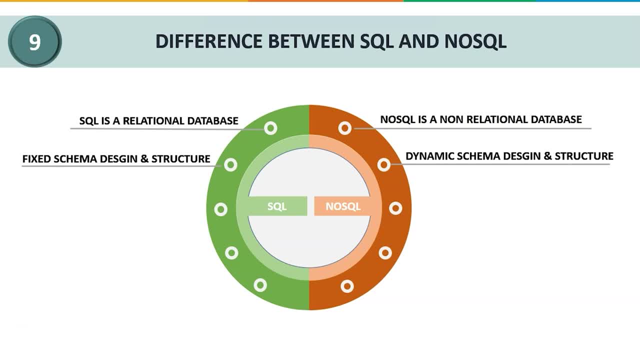 So, as we discussed, SQL has a fixed schema design and structure and NoSQL has a dynamic schema, design and structure. SQL can handle complex queries, whereas NoSQL can handle large volumes of data. Now SQL is vertically scalable. Now SQL databases support vertical scaling, which means it improves the single server by increasing RAM, SSD or CPU. 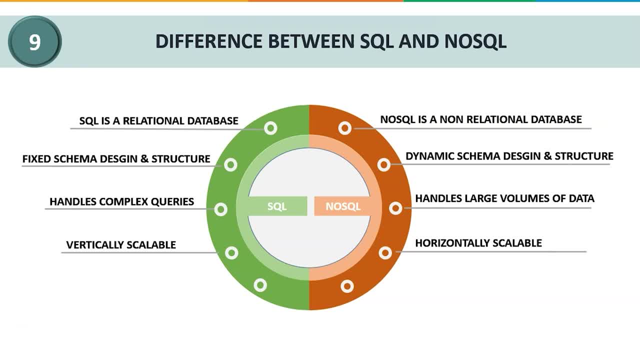 In vertical scaling we are restricted to a single system and we can improve it as much as we want, till the practical limit. Whereas in NoSQL database we can do horizontal scaling because they support distributed computing or distributed systems, In horizontal scaling we can add another node or computer for better performance. 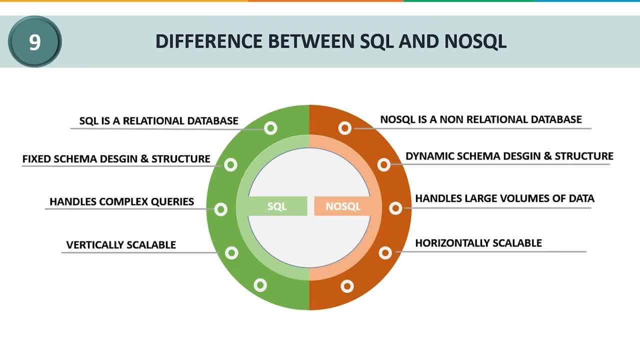 and we can add n number of such servers or nodes as per a requirement. So, as discussed, we can add as many nodes as we want and this is why we prefer NoSQL for high scalability, because there is no limit for scaling. And finally, it follows ACID properties, ie. 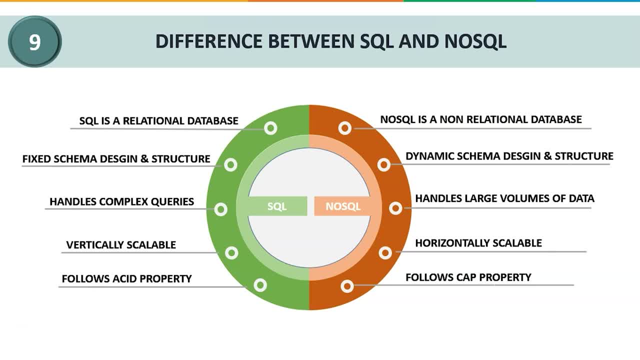 Atomicity, ie transactions should be performed at once or it shouldn't happen at all. Consistency, ie the state of a database should remain consistent before and after the transaction. Isolation, ie one transaction shouldn't affect another transaction and should be independent. 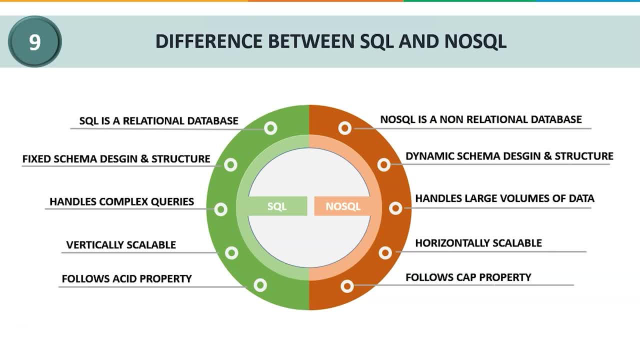 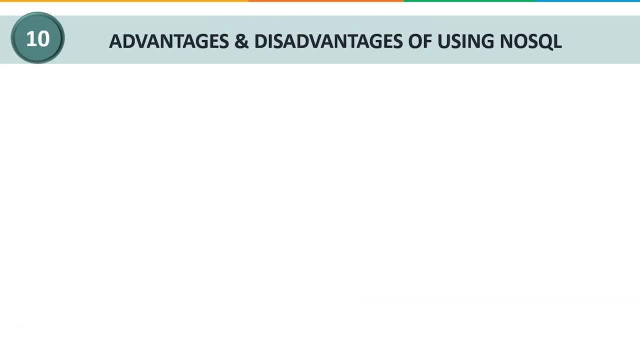 And lastly, durability- ie successful transaction- should be reflected even if there is any system failure, Whereas the NoSQL follows CAP property, ie consistency, availability and partial tolerance. Let us now discuss some advantages and disadvantages of using NoSQL. 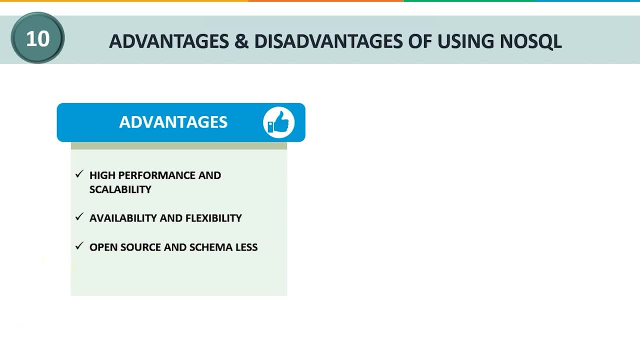 Firstly, let us discuss about the advantages. NoSQL provides high performance and scalability, and it also has a lot of availability and flexibility. It is open source and it is schema-less as well, ie you can directly download the NoSQL databases from the internet, unlike some commercial databases that are available in the internet. 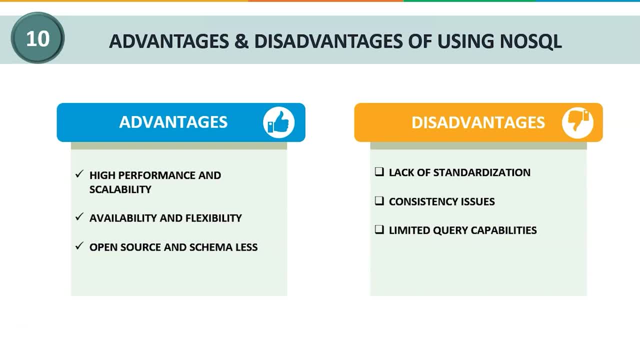 While, on the other hand, there are some disadvantages as well, ie it lacks the standardization, ie it does not have a fixed query in order to retrieve data from the databases, which result in consistency issues. And since it has all these consistency issues and does not retrieve data properly, it has a limited query capabilities. 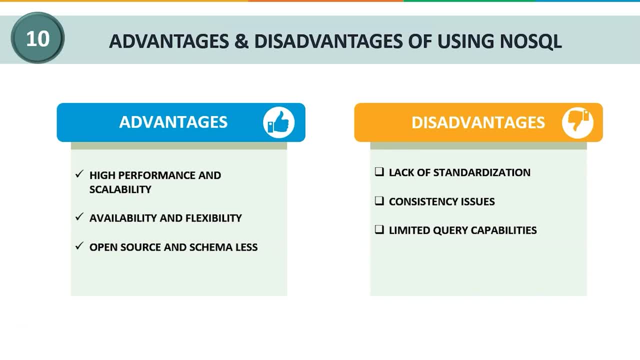 So that brings us to the end of today's session on SQL vs SQL. Thank you for watching this video. You might have a doubt that when you need to use SQL and when we need to use NoSQL. Now, SQL is easiest to work with relational databases, ie it is useful when you want to perform complex queries using various operations like join and etc. 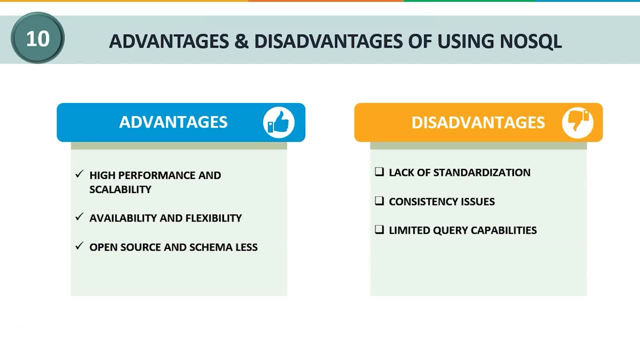 And if you want to perform quick data storage and retrieval operations, you can use SQL, Whereas you can use NoSQL if you are designing a distributed system and if you want a hierarchical storage structure instead of a tabular-like structure. Also, NoSQL gives you the flexibility to create dynamic structures and can add features as you want.